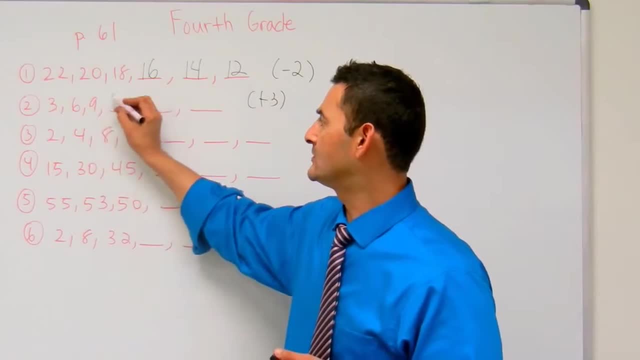 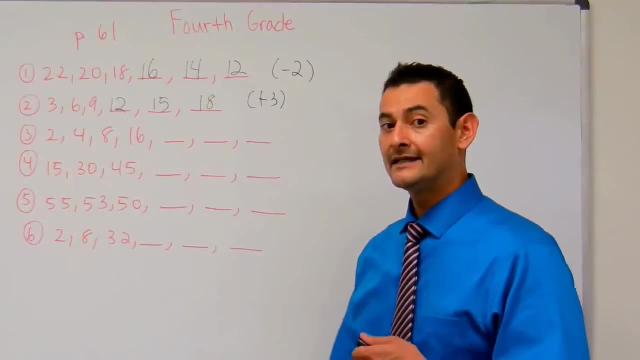 So the rule is going to be plus 3.. Now let's see: 9 plus 3 is 12, 12 plus 3 is 15, 15 plus 3 is 18, okay, Now let's take a look at number 3.. Number 3, we have 2,, 4,, 8,, 16.. So how did? 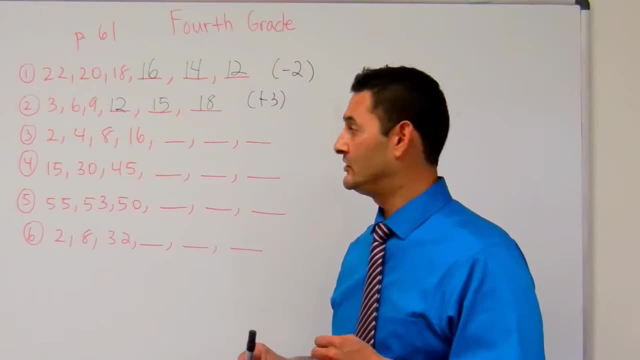 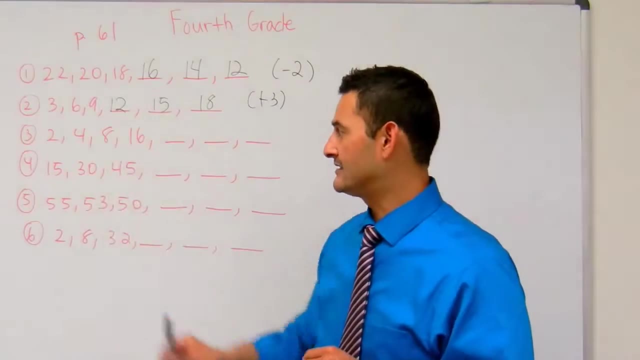 this 2 become a 4?? Well, let's try adding 2.. 2,, 3,, 4, that works. Let's add 2 to this, So 4 plus 2,, 4,, 5,, 6, that's not going to work. Let's try a different way. How about? 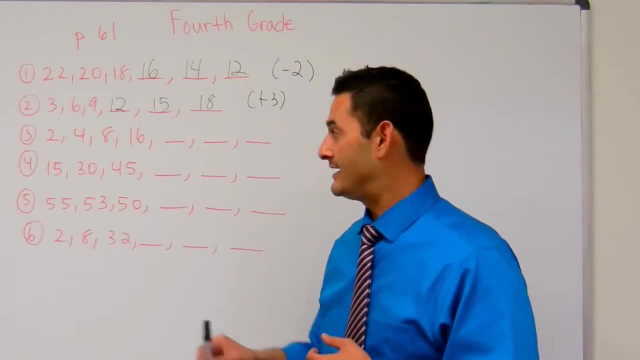 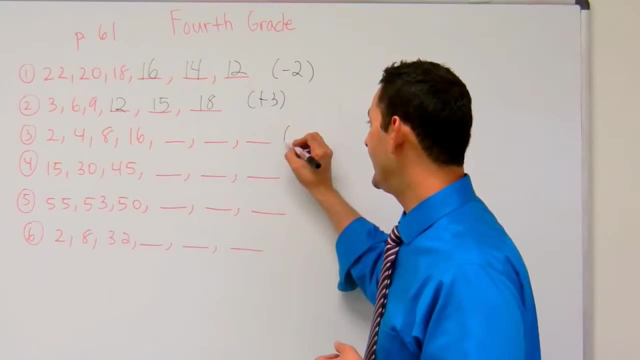 2 times 2? Is 2 times 2, 4? Yes. How about 4 times 2?? Is that 8? Yes, How about 8 times 2?? Is that 16?? Yes, So we're multiplying, so it's going to be times 2.. So 16 times. 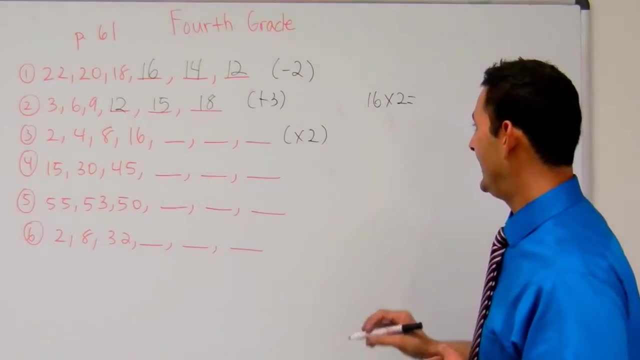 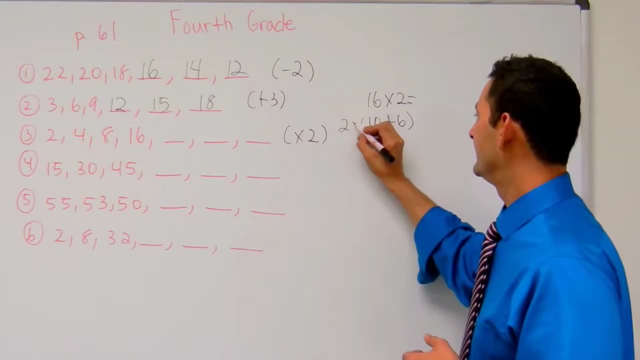 2 equals okay. Now what I can do here is I can go ahead and break this up: 10 plus 6, okay, 2 times 10 plus 6.. So that's going to be 2 times 10, that's 20, plus 2 times 6,. 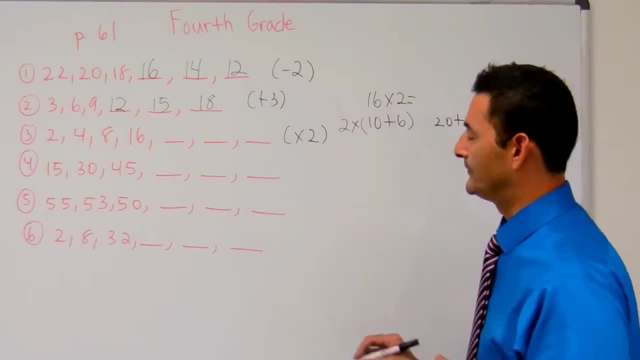 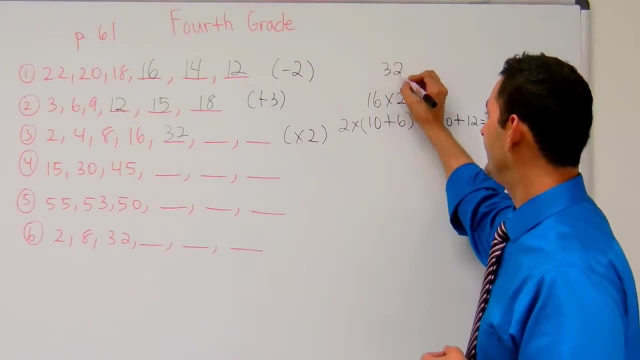 that's going to be 12,. that's going to be 32,. okay, 32 goes there Now. 32 times 2, okay, I'm going to go ahead and do that right there: 32 times 2.. I can. 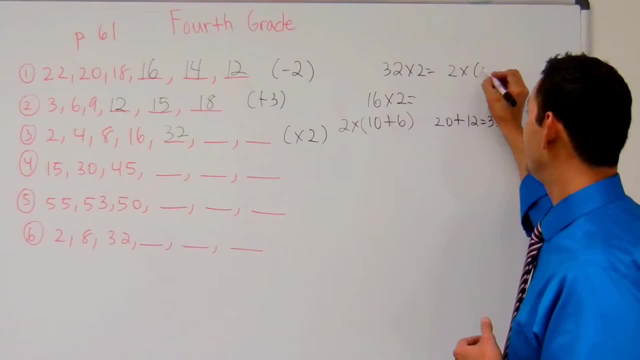 break that up using the distributive property, I've got 2 times 30 plus 2 equals 2 times 30, that's 60, plus 2 times 2 is 4, that's going to be 64,. okay, Now I'm going to go. 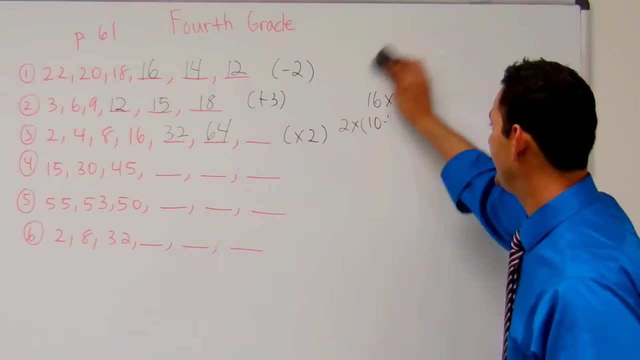 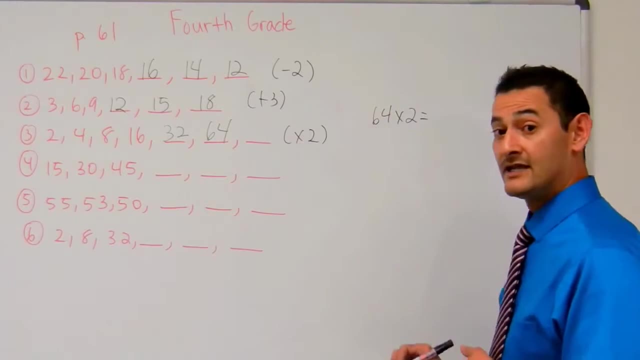 ahead and I'm going to erase a little bit. okay, So we have space. Now let's take a look at 64 times 2.. I've got 64 times 2 equals. I'm going to use the distributive property again. okay, 2 times. 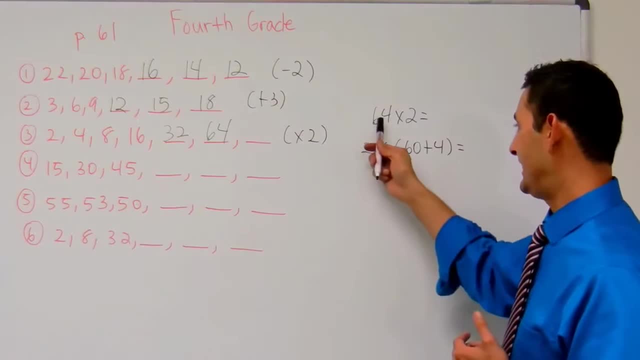 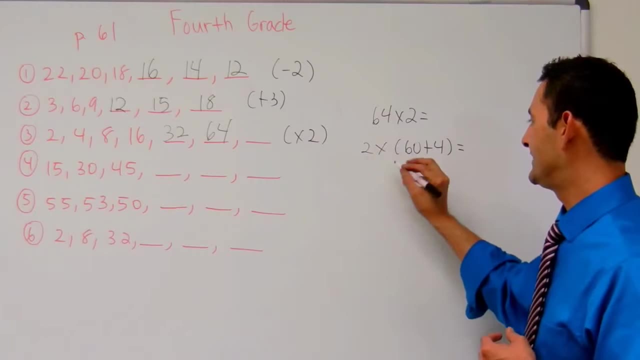 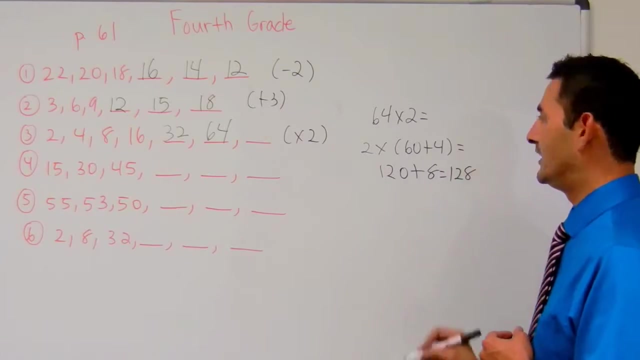 60 plus 4 equals That's: 64 is 60 plus 4, right, That's correct. So 2 times 60, place value: 2 times 6 is 12, add the 0, plus 2 times 4 is 8, that's going to equal 128.. Now let's. 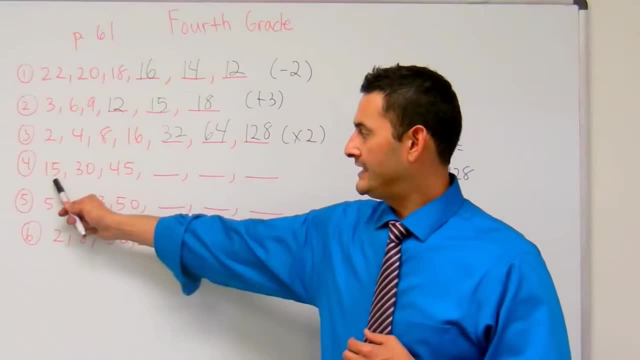 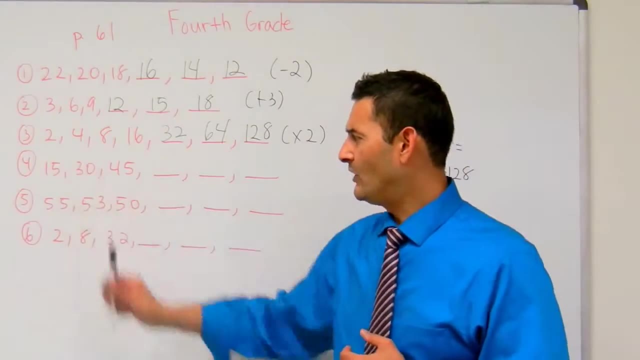 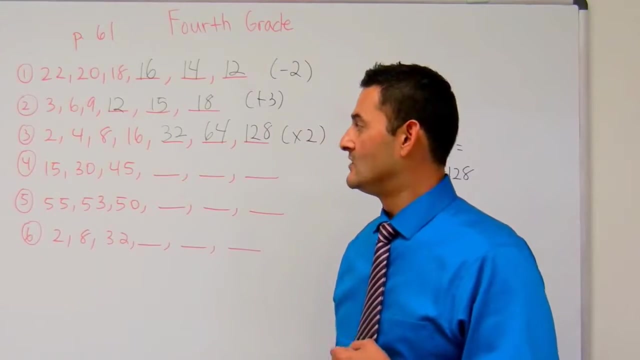 take a look at number 4.. I have 15,, then it became 30,, then it became 45. Well, if I add 15 plus what equals 30? Okay, Here I've got 110, and I've got 51, so let's double it. So 15, 110 would be 25,. 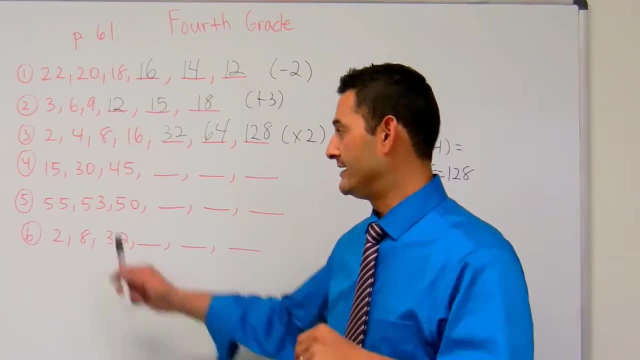 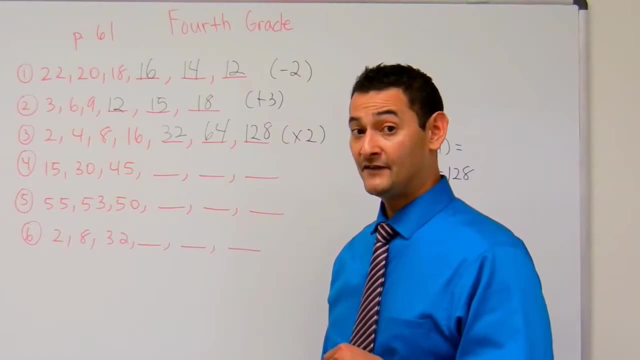 5 more: 26,, 27,, 28,, 29,, 30. So that's 30,. okay, So we have plus 15 here. Is that plus 15 here? 30 plus 15, does that equal 45?? 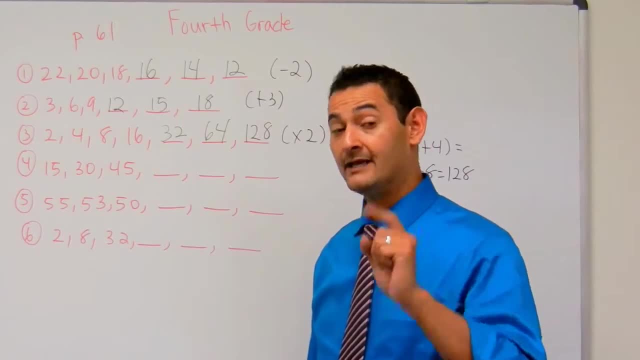 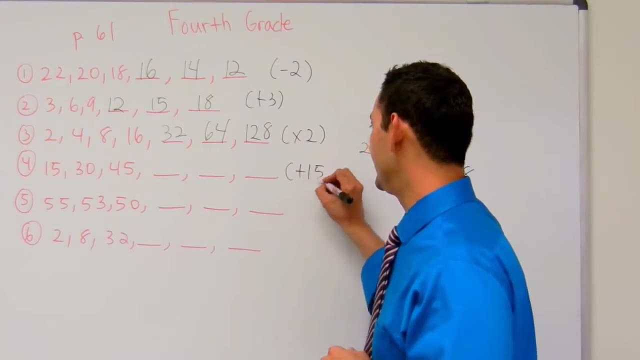 Well, let's see 30,, 110,, 30,, 40,, 5 more 1s, 41,, 42,, 43,, 44,, 45. Yes, so this rule is going to be plus 15.. 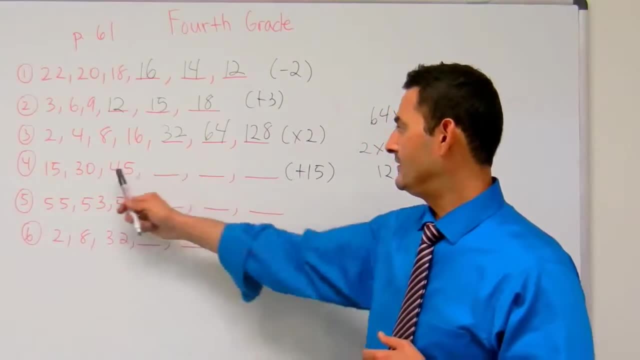 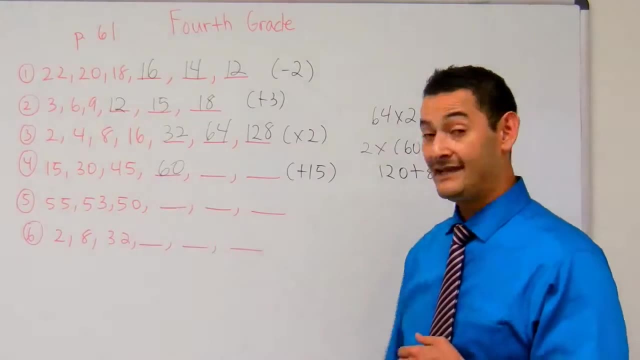 So let's just add 15.. 45 plus 15,, 110,, 55,, 5 more 1s, 60.. 60 plus 15,, 110,, 70 plus 5 more 75.. 75 plus 15,, 110,, 85.. 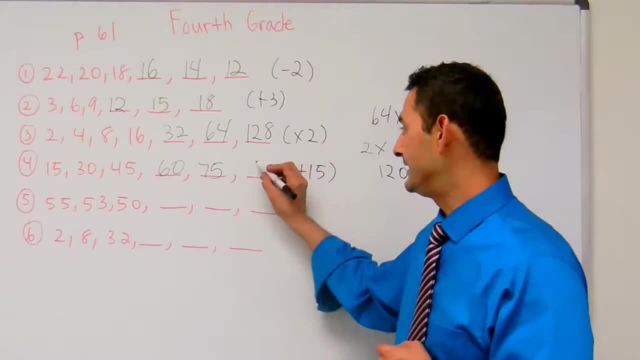 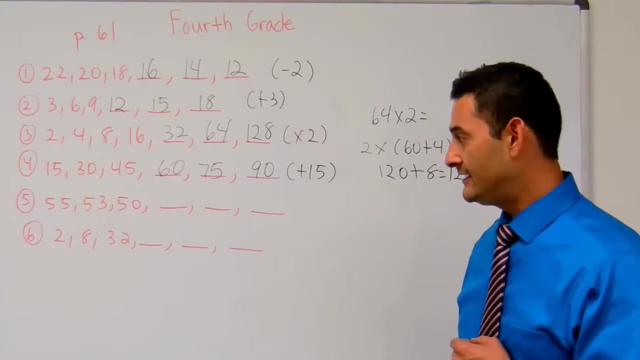 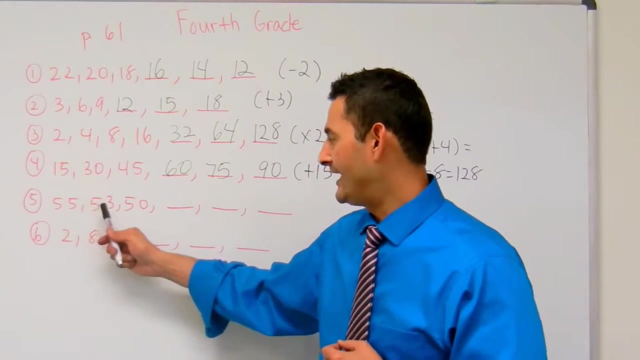 Okay, So we have 55 plus 5 more 90.. There you go. Now let's take a look at number 5.. Number 5 says 53, then 50,. no, I'm sorry, 55, then 53,, then 50.. Hmm, let's see 55, I got 2,. 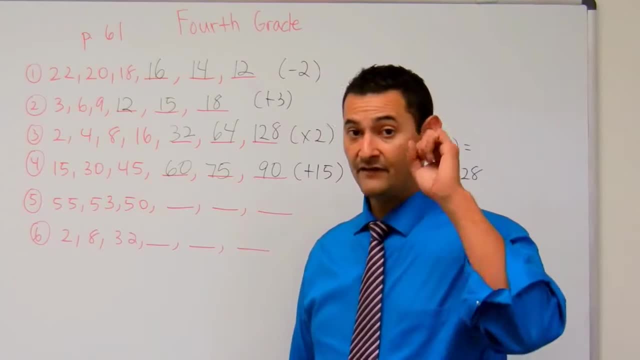 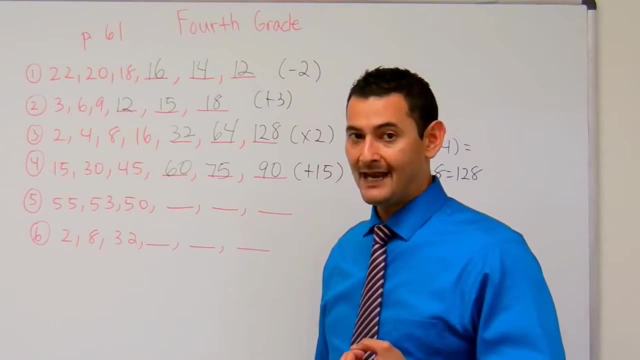 53 by taking away 2.. 55,, 54,, 53,, that's minus 2.. Here I've got 53, and then it became 50. What happens there? 53,, 52,, 51,, 50.. 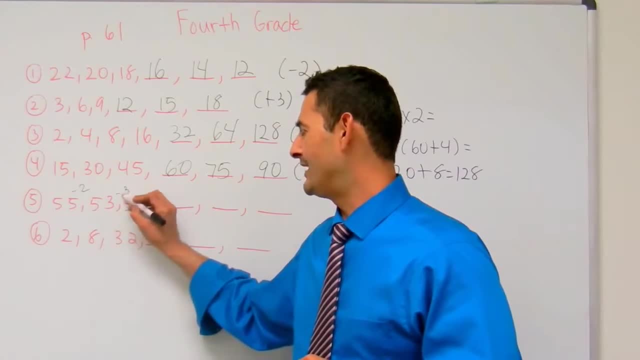 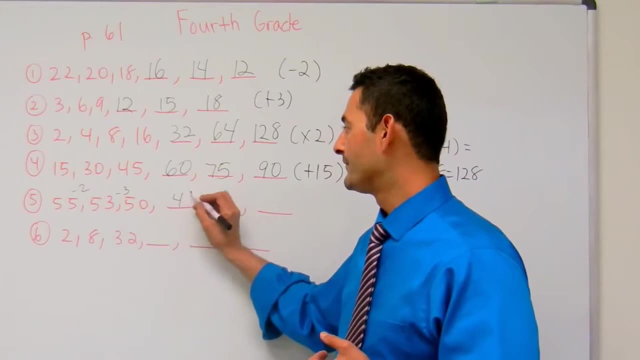 So here I subtracted by 2.. There, I subtracted by 3.. What do you think I need to do now? Subtract by 4.. Okay, so, 56 minus 4, 46. Now I'm going to subtract by 5.. 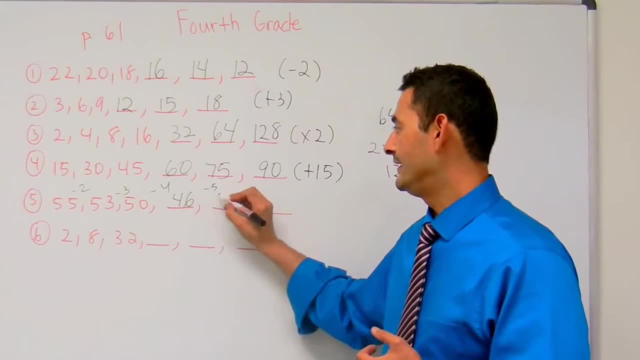 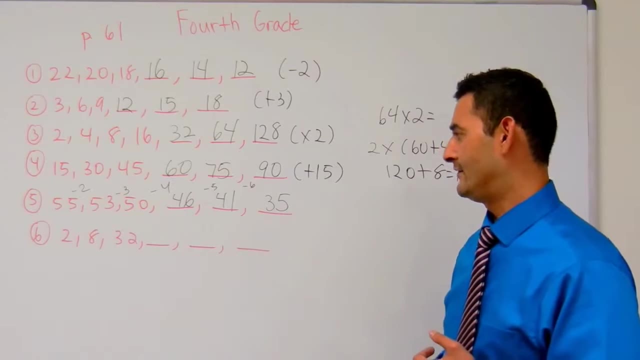 46 minus 5 equals 41. Now I'm going to subtract by 6.. 41 minus 6, that's going to be 35.. Okay, This one's a tricky one, boys and girls, and there's going to be some tricky ones in your hybrid math workbook, okay. 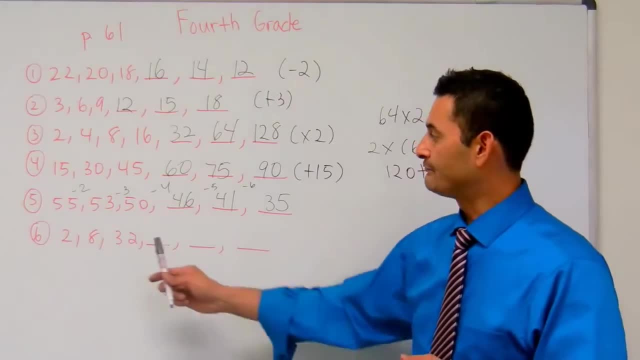 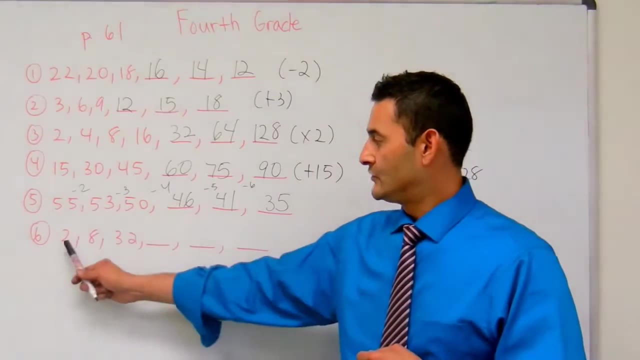 I'm not going to lie to you, But just go ahead and do the best you can. Number 6 is. 2 became 8, then 8 became 32.. 2 plus 6 is 8.. 8 plus 6 is 14.. 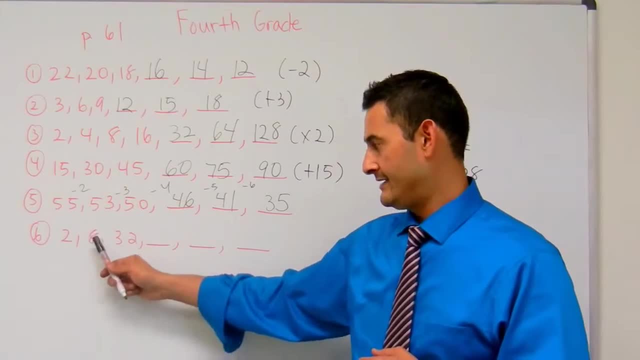 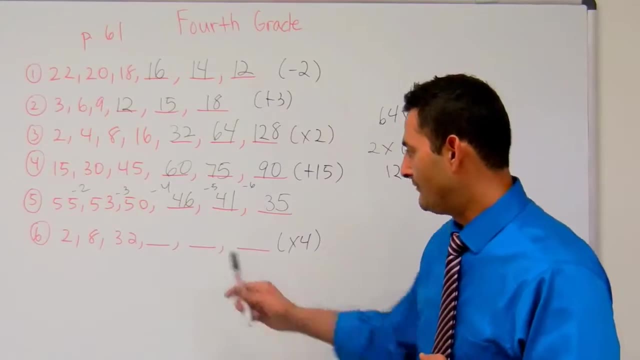 That's not 32.. 2 times 4 is 8.. 8 times 4 is 32.. That's going to work. So here I'm multiplying by 4.. So if I multiply this by 4, again I can use a scratch piece of paper. 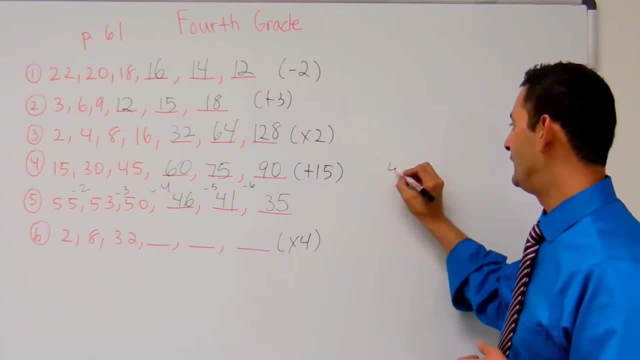 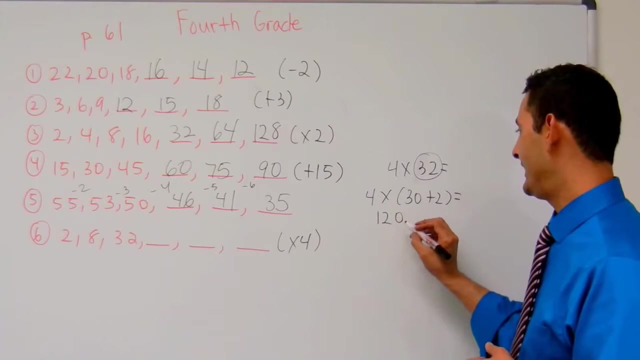 I'm going to use a distributive property of multiplication. So I'm going to do 4 times 32 equals. So I'm going to break this piece up. It's going to be 4 times 30 plus 2 equals, 4 times 30, 120,. 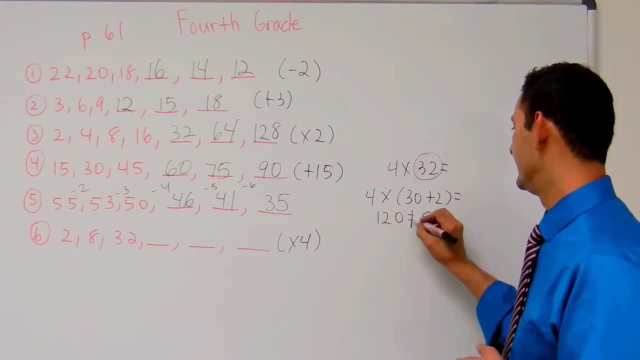 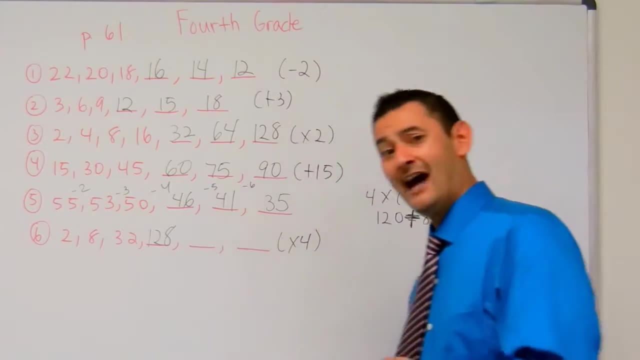 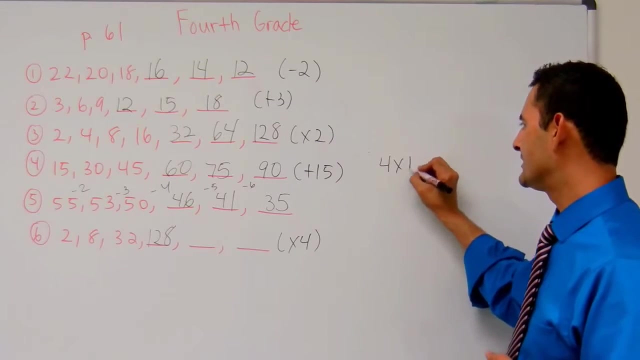 equals 4 times 2 is 8.. Okay, 120 plus 8 equals 128.. Okay, And now these numbers are going to get large. okay, Because we're multiplying by 4.. That's okay. So here we have 4 times 128 equals. 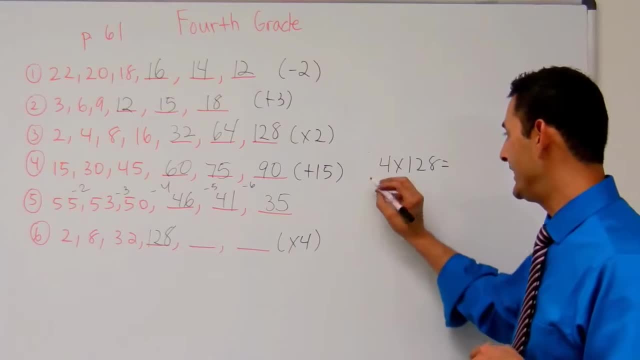 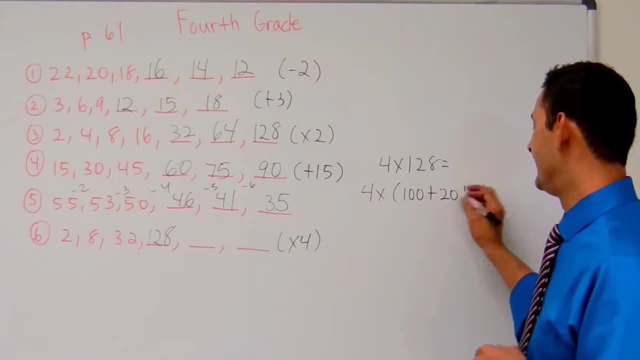 So here, what I'm going to do is I'm going to use the distributive property again. Here I've got 4 times, That's 100.. Plus That's 210.. That's 20.. Plus is 8.. That's just 8 ones. 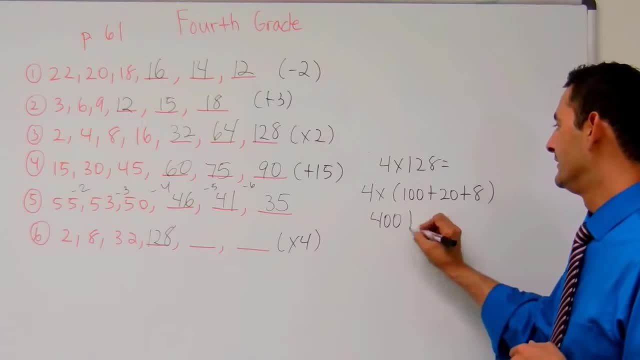 So now 4 times 100.. That's 400.. Plus 4 times 20.. That's 80.. Plus 4 times 8. That's 32 equals. Okay. So now what I can do is I can go ahead and do 400 plus 80 plus. 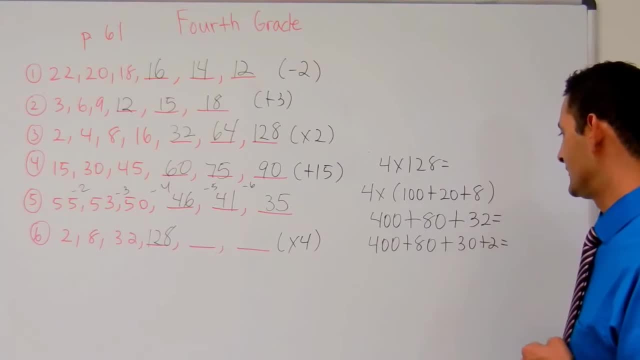 I'm going to go ahead and break that apart. 30 plus 2 equals. So here I've got 400 plus 80 plus 30.. That's 480 plus 30 plus 2 equals. I need 2 bundles of 10 to make 500. 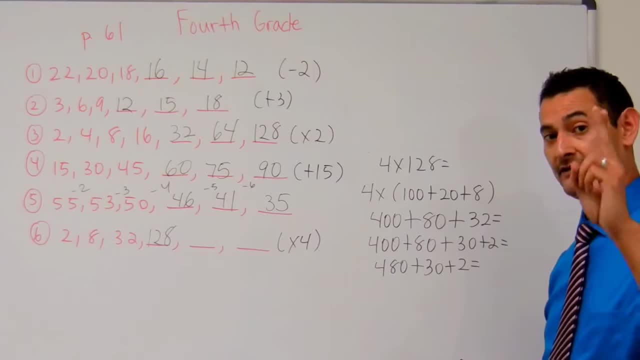 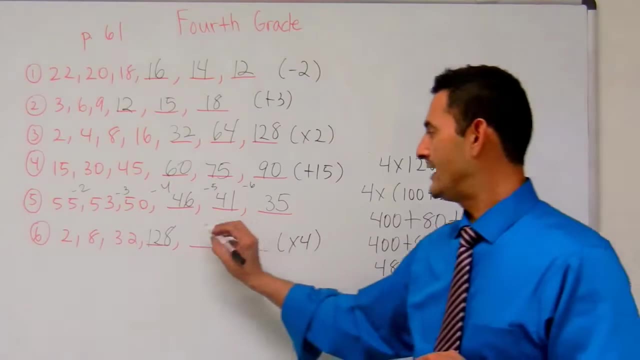 480 plus 30.. 490 plus 30 plus 2 equals 510.. 510 plus 2 equals 512.. So that's going to be 512.. Okay, And now let's go ahead and take a look at 512 times 4.. 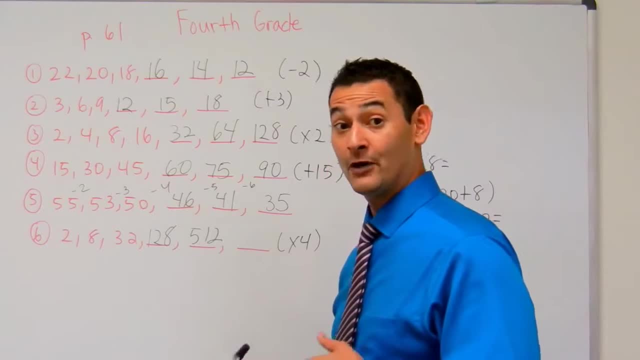 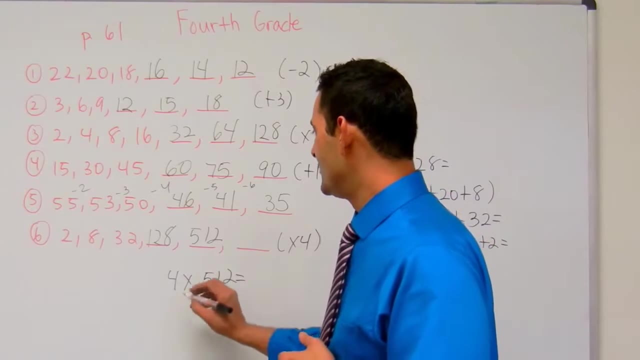 My goodness, These numbers are getting large, aren't they? It's a good thing. we know the distributive property and place value, So let's go ahead and do 4 times 512, equals Okay. So here I'm going to do 4 times 500.